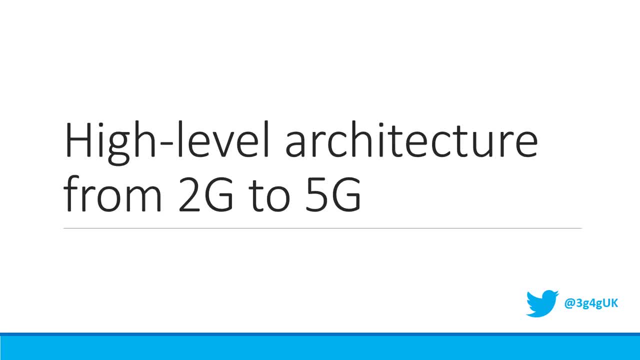 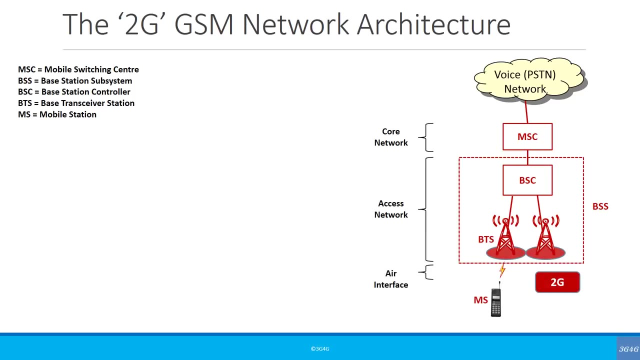 Hello everyone. in this video we will look at a very high level architecture all the way from 2G to 5G. I am intending this for this to be a very small video, So let's start with 2G. GSM network architecture. Most of you would be aware that GSM was initially 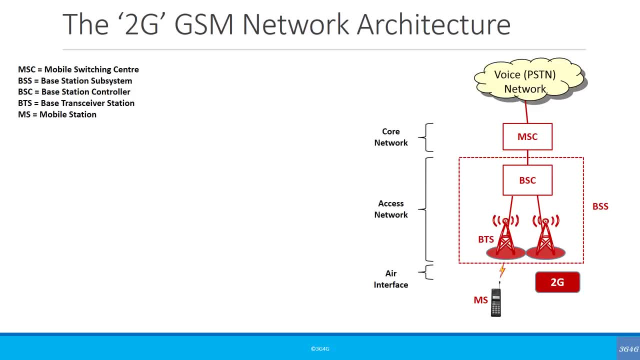 designed only for voice. There was no intention for data, and even SMS came much later, But GSM, as I said, was designed just for voice. Now, the original GSM architecture consisted of the access network, which is the BSC and the BTS, and this, so the base station controller. 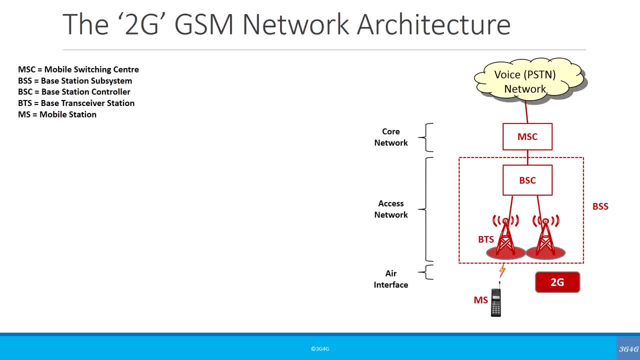 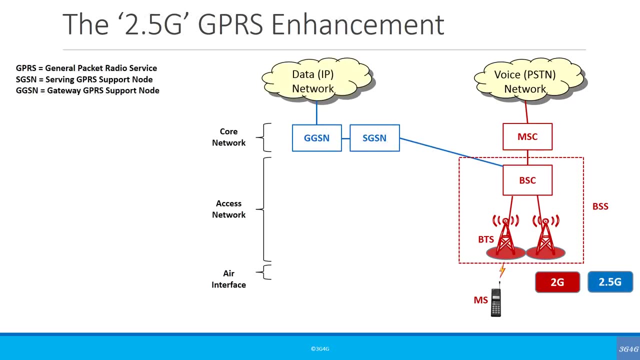 and the base transceiver station And together they were called as the base station subsystem. Okay, you had the mobile station and you had the MSC mobile switching center for voice calls. In 2.5G GPRS enhancement the data part was added to the voice part, so the data core network. 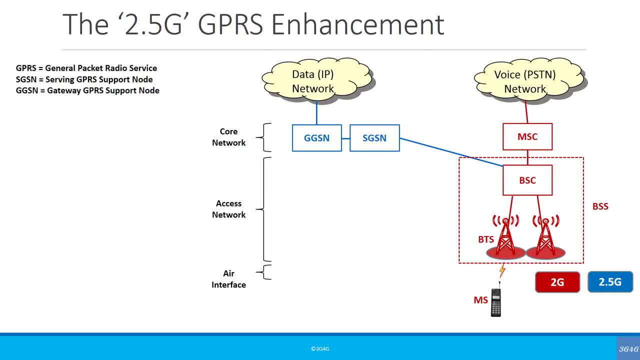 the MSC was the circuit switch core and the packet switch core was added, which consists of SGSN and GGSN, the serving GPRS support node and the gateway GPRS support node. Everything else remained the same. Of course, the BSC and the BTS had to be enhanced to handle the new data network, the packet. 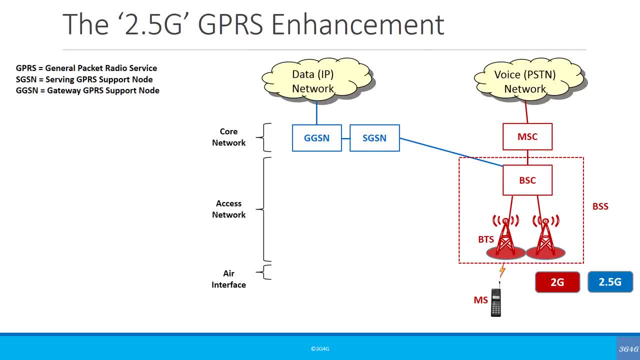 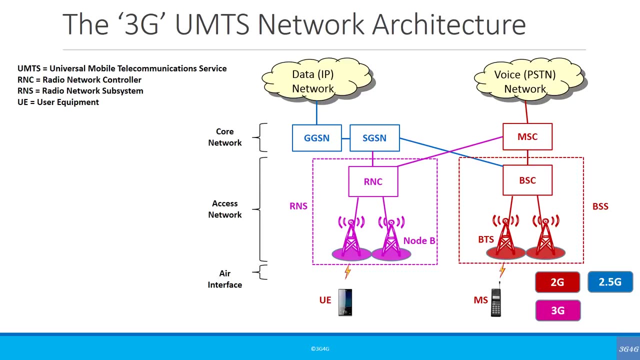 switch core and the mobile had to handle the packet switch part as well, But otherwise, in theory, everything else remained the same. 3. The 3G network built on top of this 2 and 2.5G network, So it retained the same circuit switch and the packet switch core network. 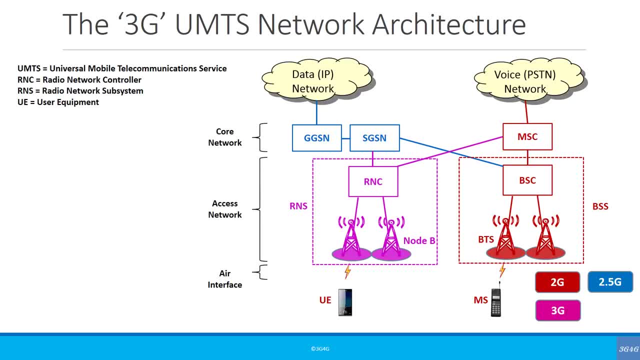 But we had the new access network, So the RNC, the radio network controller, was equivalent of the base station controller and the node B was equivalent of the base transformer. So the RNC was equivalent of the base station controller and the node B was equivalent of. 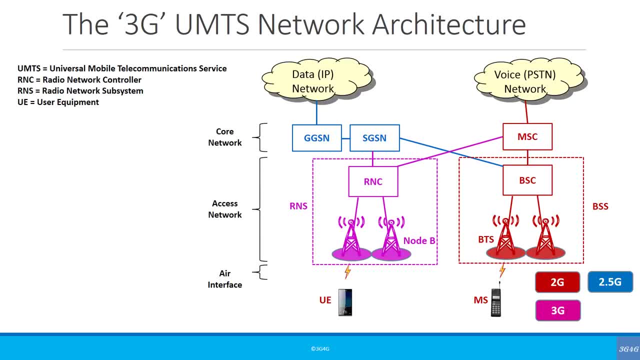 the base transceiver station BTS. Now, I often get asked a question about why is this called node B? Well, initially people could not come up with a better name, a replacement name, for BTS, So they called it a node B- like you know, the equivalent of BTS- and the intention was to 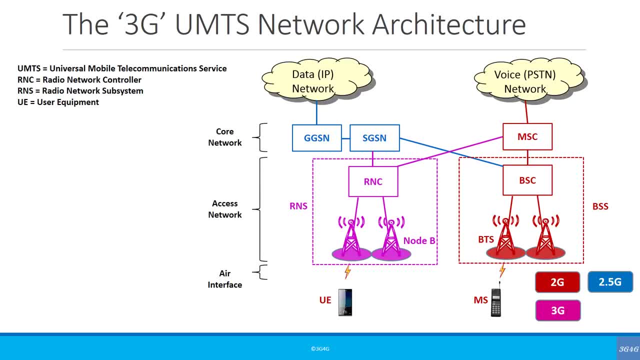 actually come up with a finalized name much later on. But then things move on and everybody is busy. So the node B name, the node B terminology, stuck 4. In the standard. so it's still called node B and you will see it evolved further on in. 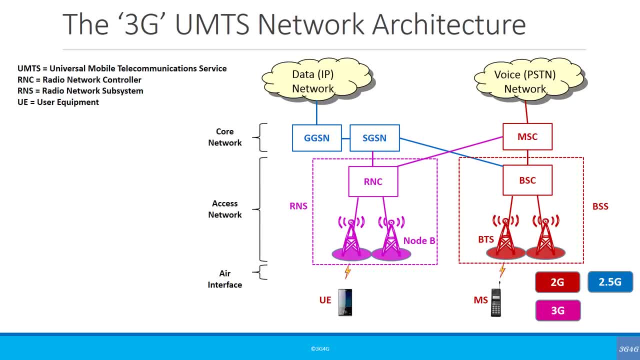 4G and even in 5G right. And one of the other changes is, instead of a mobile station, now from 3G onwards, the device is called the user equipment. I have done a separate tutorial on this particular topic, which you can actually find on YouTube. 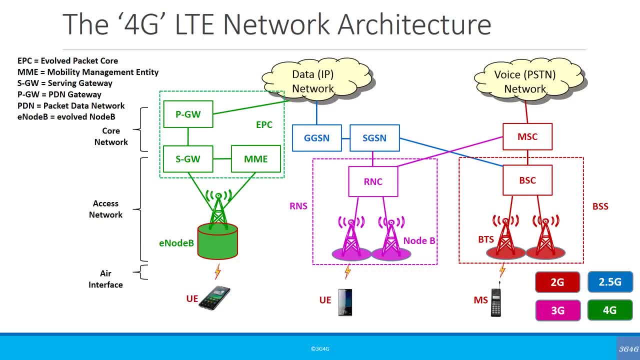 5. In 4G We do not carry on the circuit switch core, So we only maintain the packet switch part right. but also a new packet switch core network was invented for 4G. As you can see, you have the UE, you have the evolved node B. 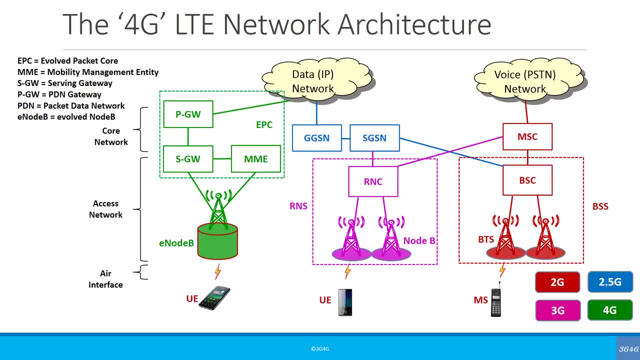 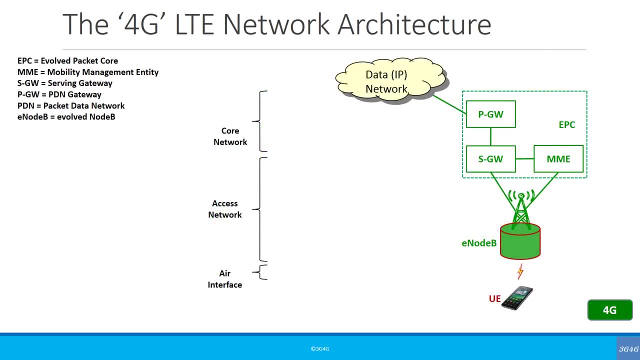 Then in the core network you have MME, which handles the signaling part, and the serving gateway, Which handles the the data part 6.. Now, if you look at the 4G network, architecture by itself right, because the main intention when 4G was designed was to actually get rid of the legacy architecture. 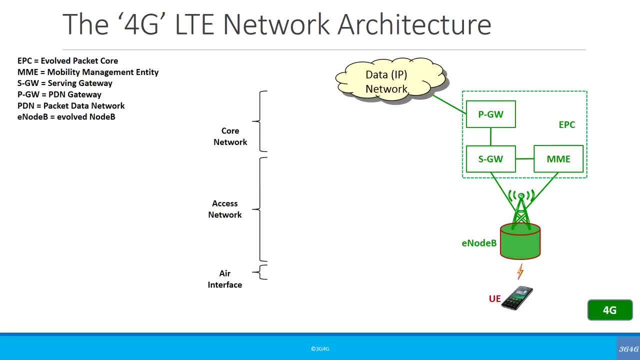 So there is no circuit switch core, it's only the packet switch core. 7.. In the phase 1. Phase 1 of 5G network, which is being standardized at the moment as we speak, The new, evolved, further evolved eNodeB is called the gNodeB. 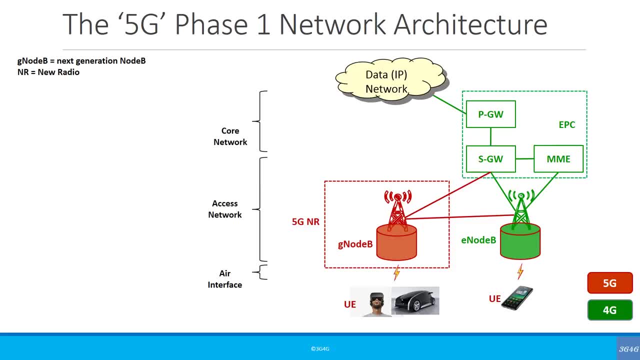 G stands for next generation node B and in the phase 1 the gNodeB will work with the existing evolved packet core EPC. So the eNodeB will do the signaling part and the gNodeB will mainly be used for the data part. 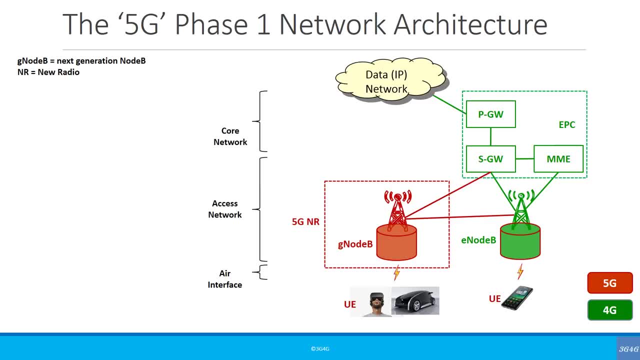 So think of it as like a. the gNodeB will be doing some sort of like a carrier aggregation in conjunction with eNodeB. It's not exactly carrier aggregation, but you can think of it like that. 8. Later on, when the next generation core network is ready, 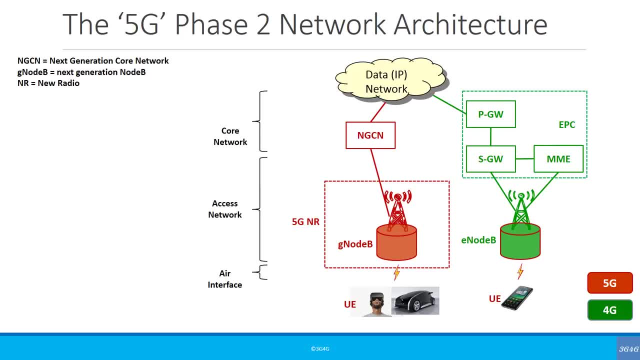 So even though I say phase 2, it may not necessarily be phase 2. So when the next generation core network is ready, 9. The gNodeB will work through the next generation core network and in some cases the existing 4G eNodeB will work through the existing evolved packet core. 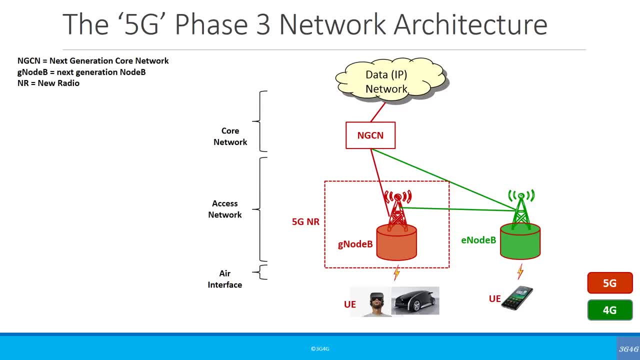 10. Later on, even though I say phase 3 later on, the 4G access network, the eNodeB will work with the next generation core network 11. So in the previous video I saw in phase 1 the gNodeB works with the evolved packet core. 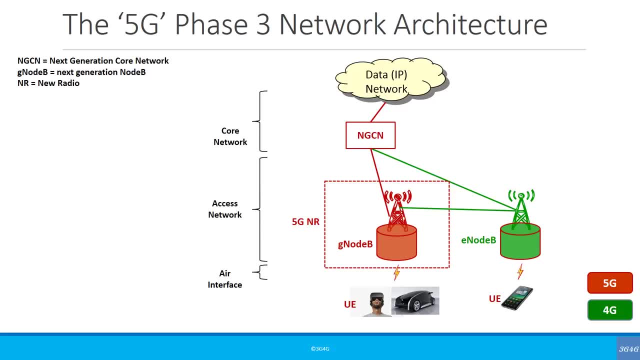 right In later on. so even though I refer to it as phase 3 in the standards, there is no phase 3.. So this is just my terminology, 12. But later on, eNodeB will work in conjunction with gNodeB, and it will, they will basically. 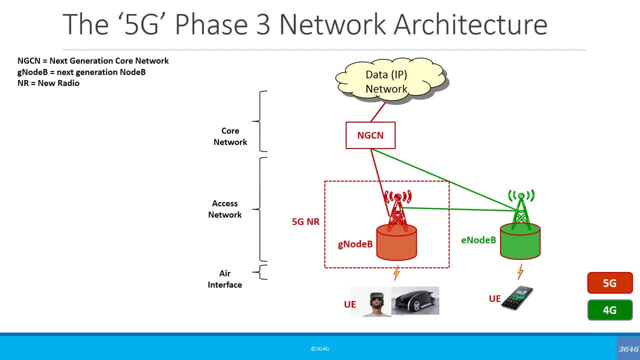 eNodeB will connect to the next generation core network, 13. So for the older devices which only support 4G, 14. They will continue to work through eNodeB, but the newer devices, which will support 5G, 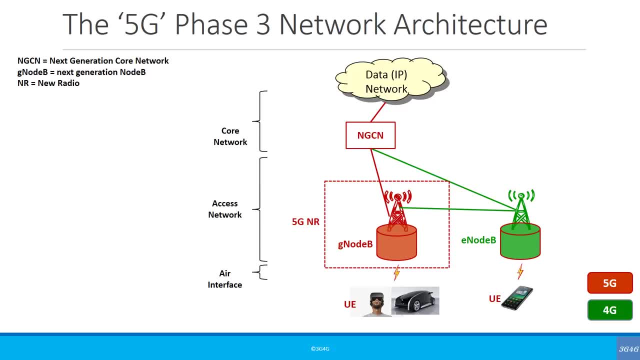 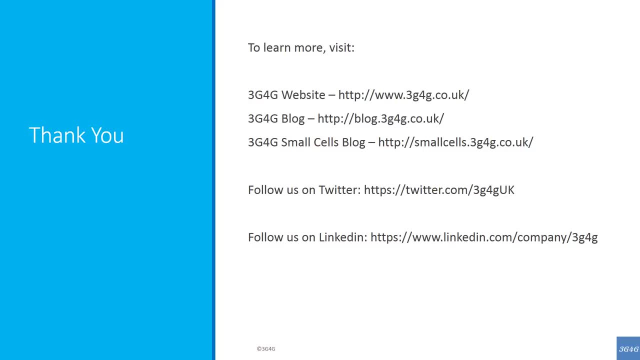 they will work with gNodeB and eNodeB. And that's about it: a very short and sweet overview of architectures all the way from 2G to 5G. I hope you enjoyed it and if there are any comments, please feel free to leave the comments. 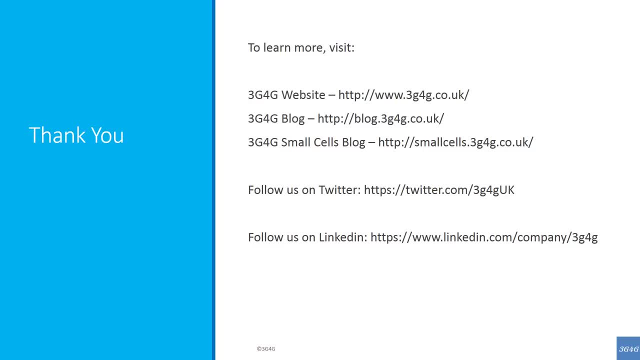 in the comment section. Thank you, Thank you.